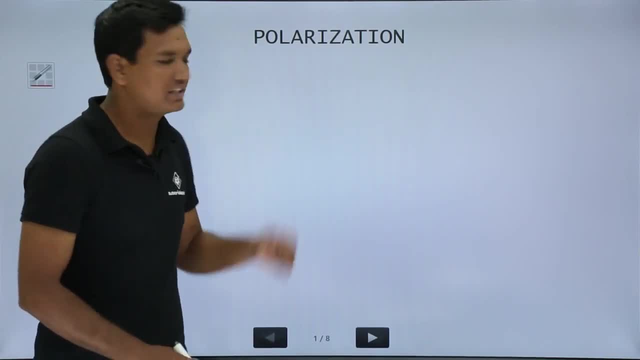 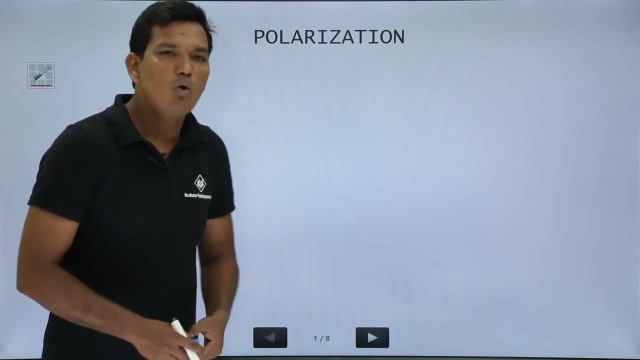 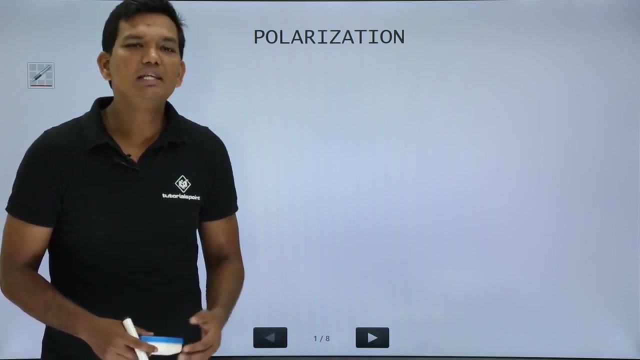 In this class we'll discuss about polarization. We'll try to understand what is a polarization. It is one of the important topics of electromagnetics. Now, when we say polarization, there are three types of polarization: Linear, circular and elliptical. We'll see each one by 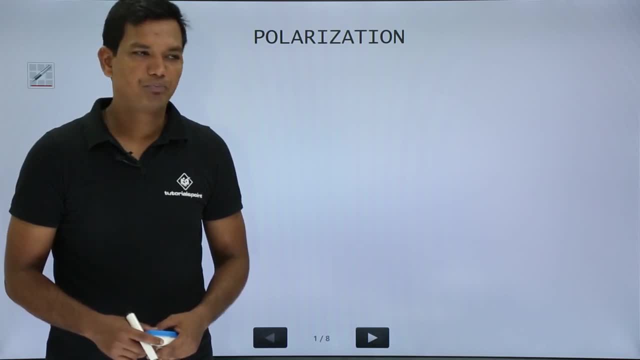 one. I'll try to understand. what do you mean by polarization? See, when I say polarization, it is nothing but the variation of electric and magnetic field component. So let's try to understand one by one and we'll focus more on that. So let's go to the first type of polarization. 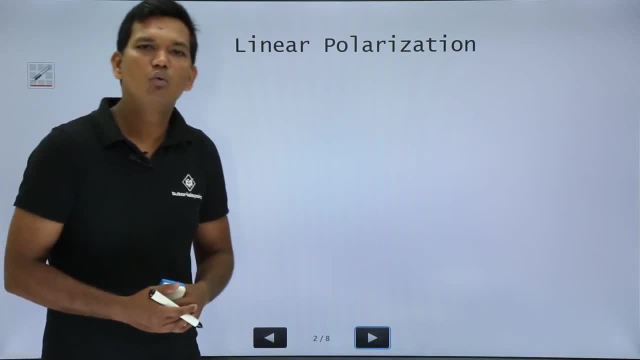 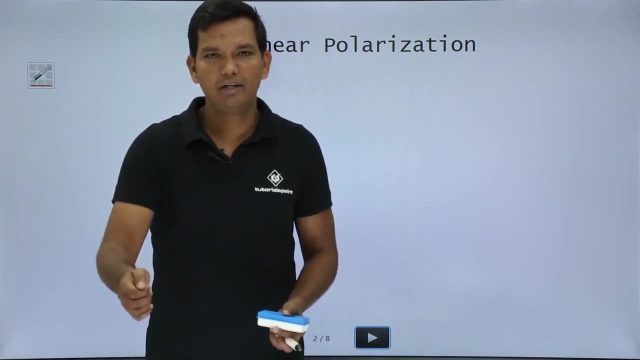 which is nothing but our linear polarization. Now, what is a linear polarization? Let's say that. I'll take one example. Let's say that I have a string in my hand. So let's say that I have a thread in my hand. What I'll do is I move the thread like this. So what will happen? The thread. 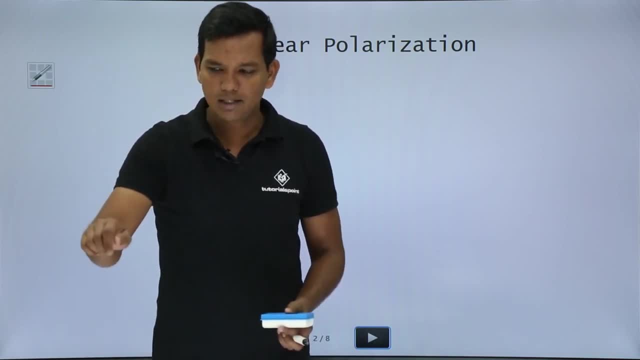 will be like a wave. So what will happen? The thread will be like a wave. So what will happen? It will be like a wave shape and it will be going up Again- same thread, If I do like this. 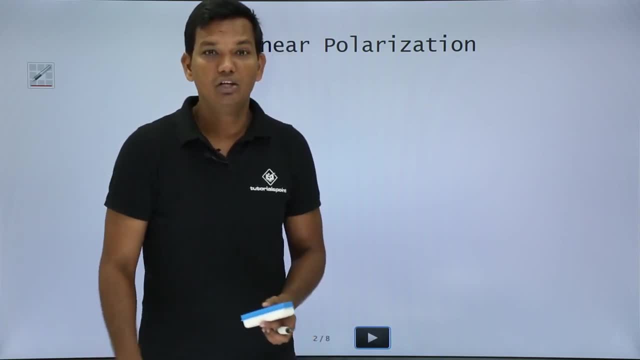 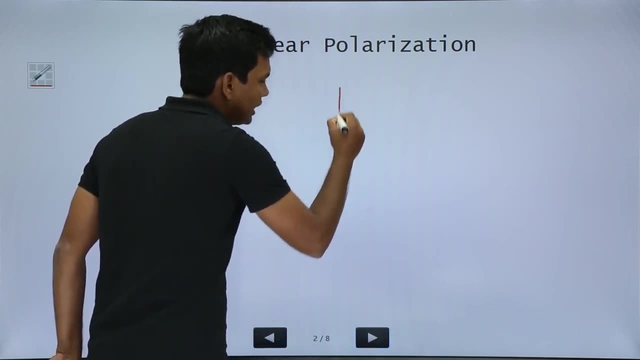 if I move very fast, the thread will go like this: This is what is happening, is the component of. so what is happening is in linear polarization is your electric field. Let's talk about electric field only. Either your electric field is varying along the, let's say, y-axis, or it is varying. 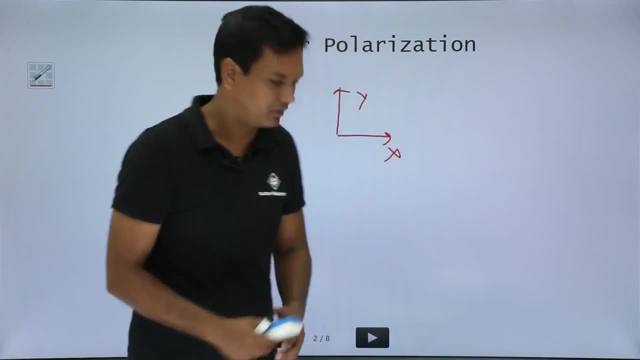 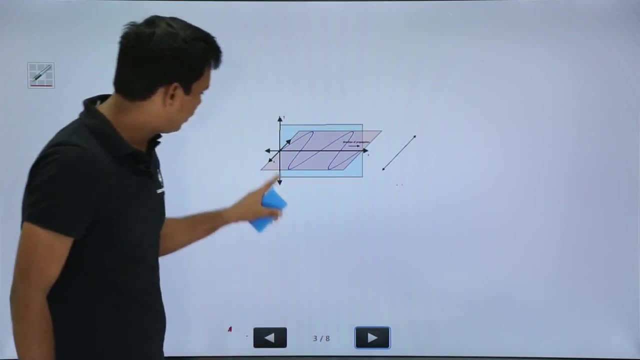 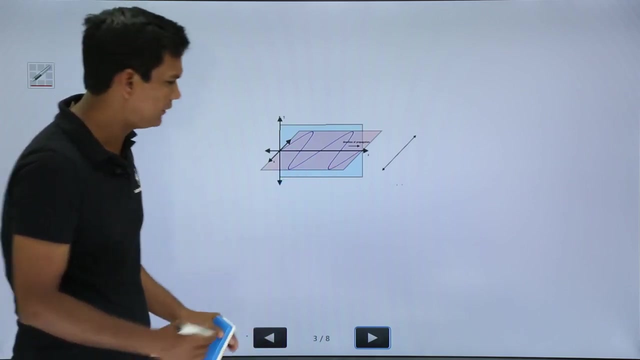 along the x-axis. Let's understand this by a figure. If you observe here what is happening is there is an e-field varying along the x-axis, right? So the variation of electric field is along the x-axis. If I try to write the equation here, how the equation will look like The equation: 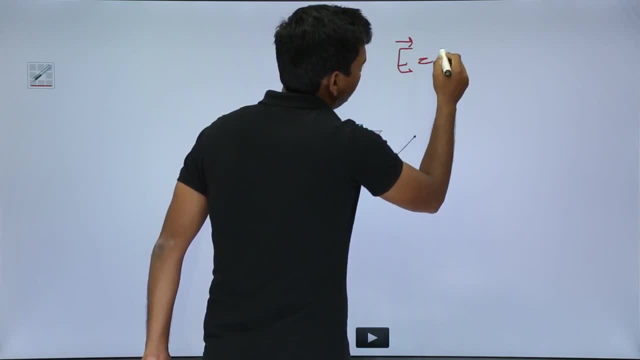 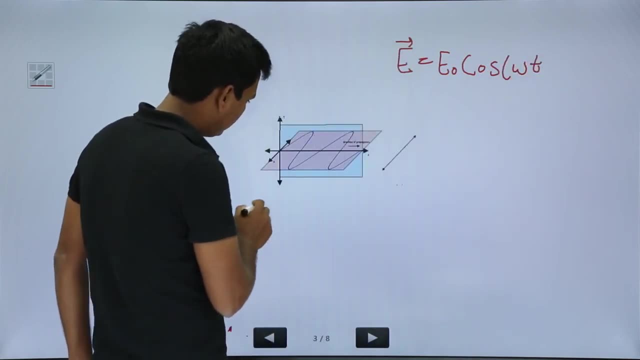 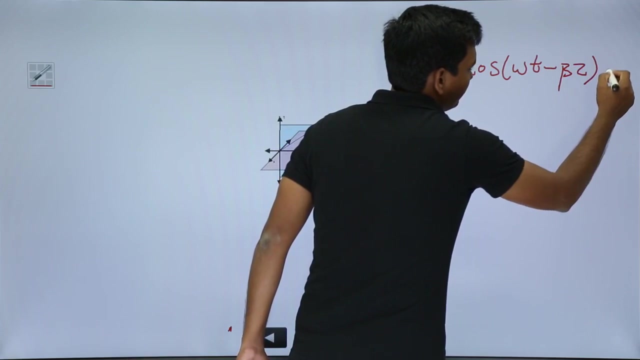 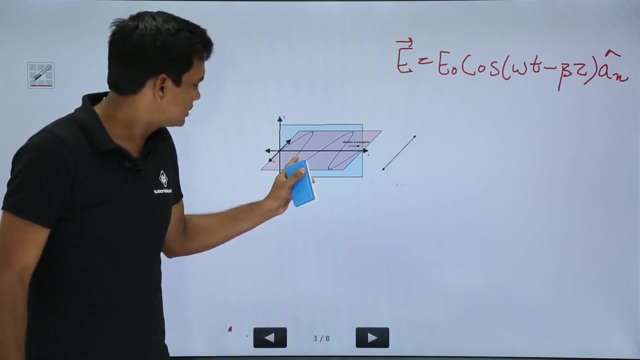 would be. e field will be nothing but e naught cos, omega t. Let's say it is propagating along the. the variation is along the x-axis and propagation is along the z-axis. So minus beta, z a, x cap. So, if you observe, I have tried to written this wave into a equation, So it is saying that. 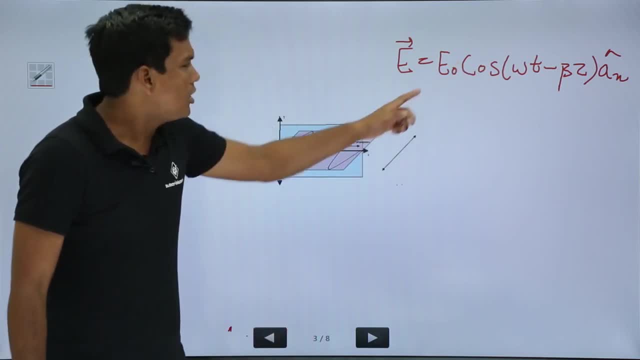 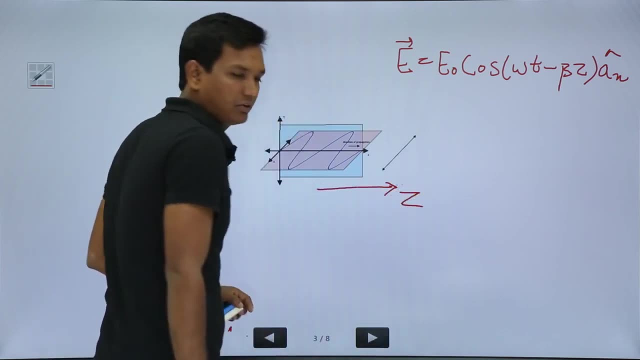 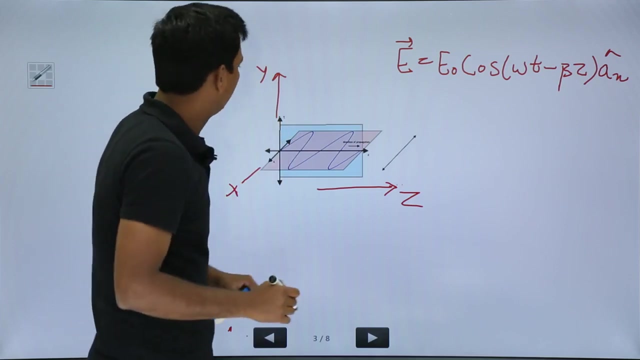 e equal to e. naught cos omega t minus beta z Minus beta z, saying that it is propagating. So the wave is propagating along the z-direction, okay, So if you observe, this is what is your x-axis right? This is what is your y-axis, right? Okay, So it is propagating along the z-direction. 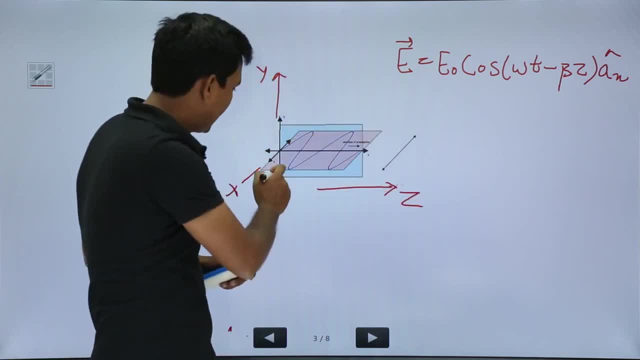 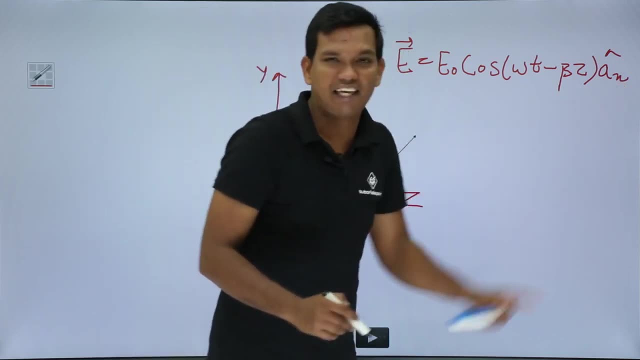 but the variation. you see, the variation is there in the x-plane right, And this is what is your x-plane right. So this is what is your x-plane. So the variation of electric field is along the x-plane right. So it has only one component, which is nothing but the variation along the x-plane. 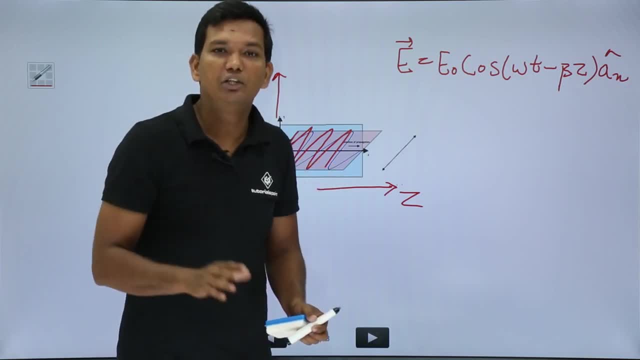 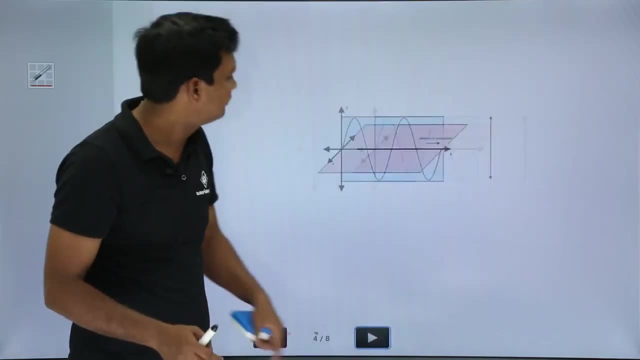 right, So this is nothing but your linear polarization, where the variation of electric field is along the one plane, right, Okay, Let us see what is the other scenario. The other scenario, if you observe, it is nothing. but now again, if you see, 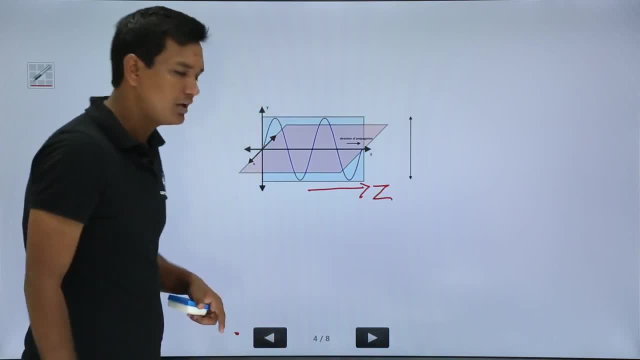 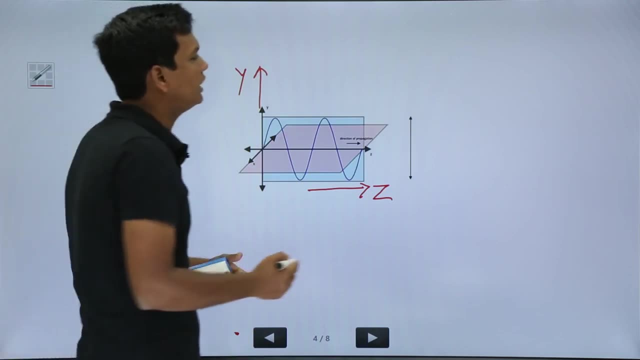 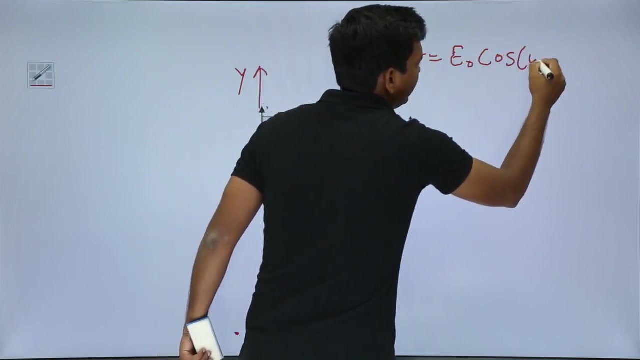 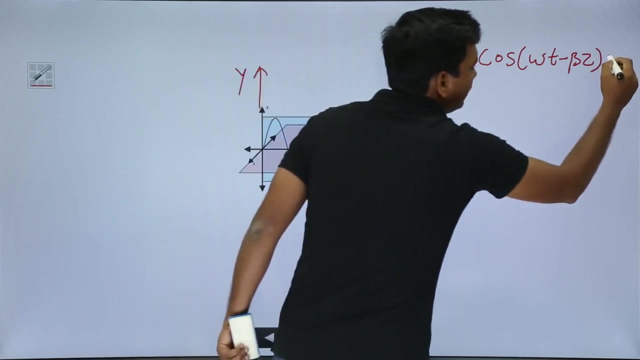 the wave is propagating along the z-direction, but the variation of electric field is along the y-direction. If I want to write the equation, how does it look? like E is equal to E naught cos omega t minus beta z, And as the variation is along the y-axis, it would be A y cap, right? 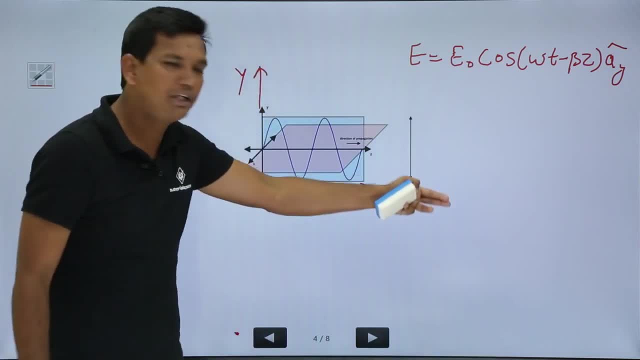 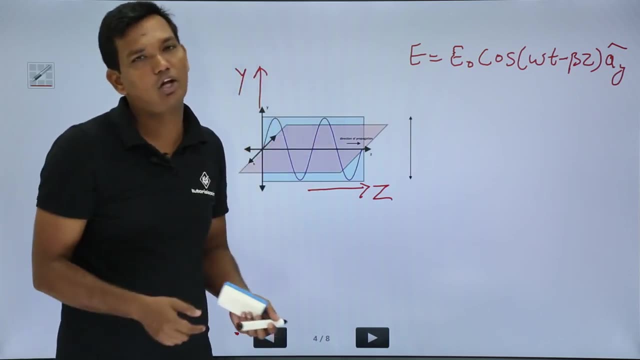 See, this is what I have written here. So though it is propagating in the z-direction, the variation is now along the y-axis, So it has one component. now, In this case, it is along the y-axis. So whenever your electric field is having 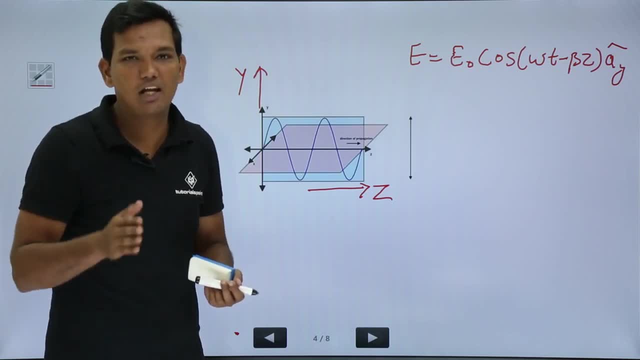 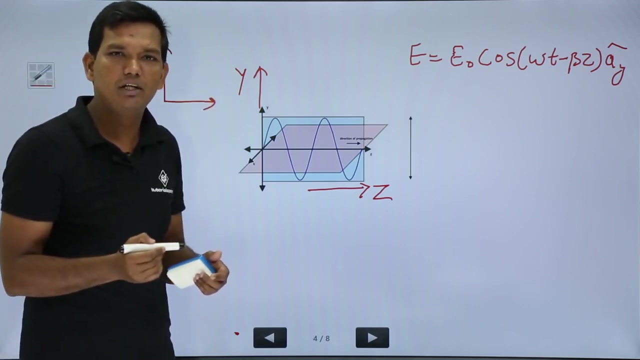 the x or the y component, or the variation is along the either x or y-axis. it is nothing but your linear polarization. Now, when you have a variation, it means if it is like this or like this, then it is a linear polarization, right. 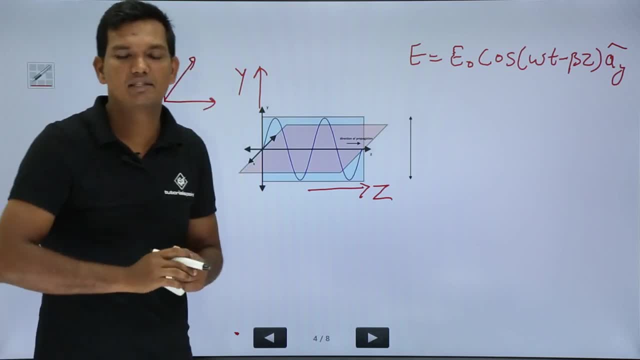 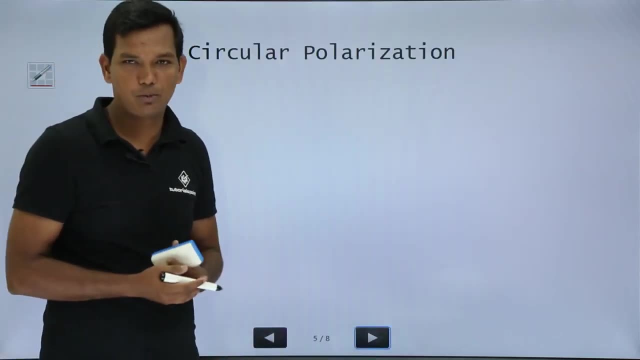 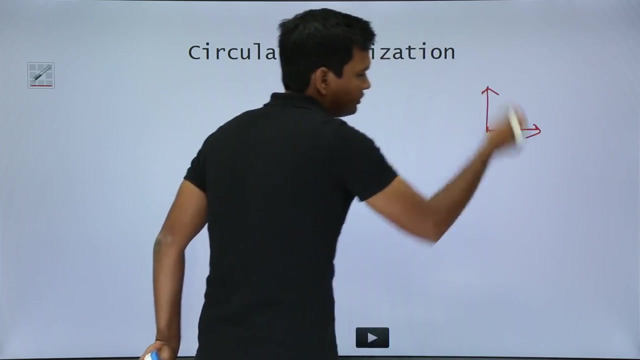 What would happen if it is something inclined to x and y-axis at some angle? right Now, that would be your next case. Let us see that. So our next case is nothing but a circular polarization. So what we said is, if it is along the x-axis or y-axis kind of this, then it is your linear polarization. But 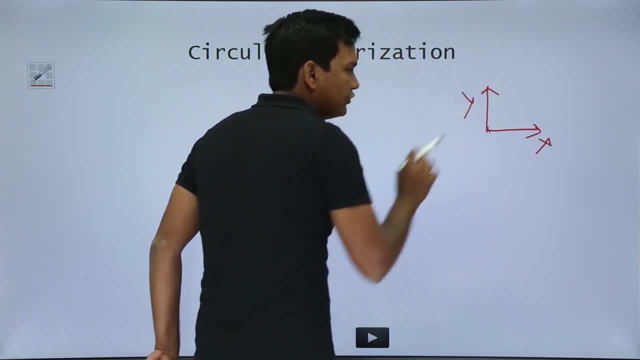 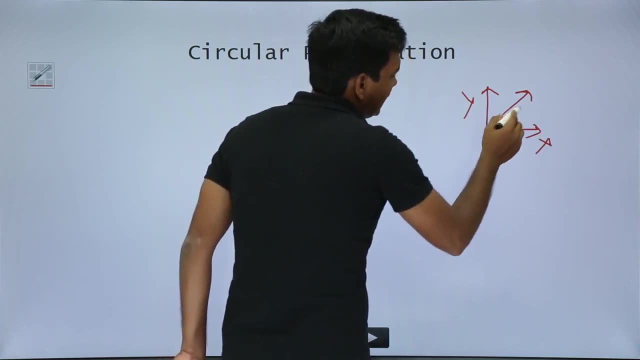 let us say that this is x-axis and this is y-axis. But if your electric field is inclined at certain angle, I do not know what is the current angle. right, Let us say that your electric field is inclined to x and y. Then in that case, what will happen If? 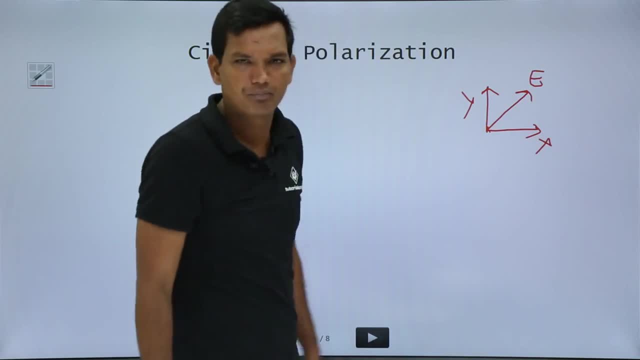 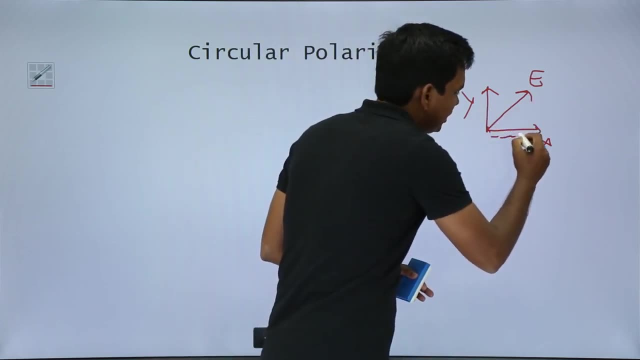 this is my e field. it will have x and y component, both right. If your electric field is inclined at some angle to the x and y-axis, it means it will have. if I break down this, it would be nothing but your. let us say that: e x cos theta. Let us say this is theta, e x cos theta. And this would. 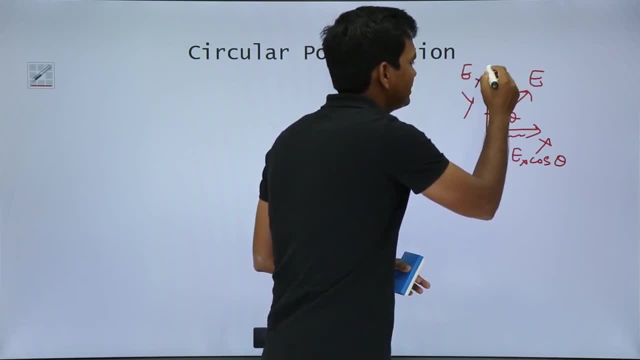 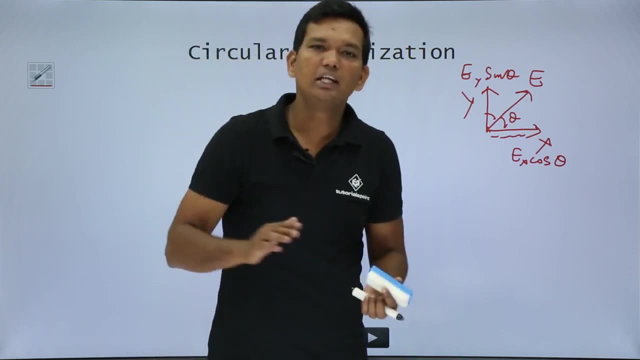 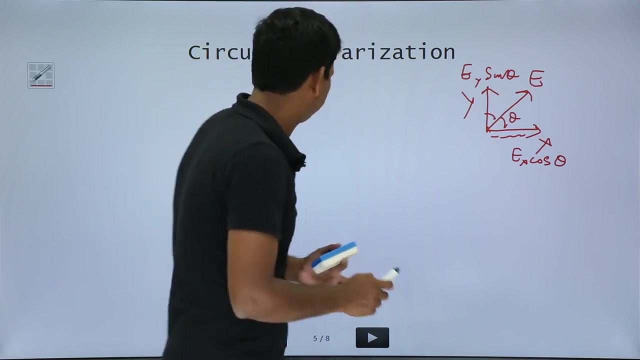 be nothing but e, y sin theta. This is how it will be if it is inclined to some plane, right? Okay, So what we said is if your electric field is inclined to some plane, it will have x and y component. Okay, So it is the same way. what will happen is, if I have some field like this and if 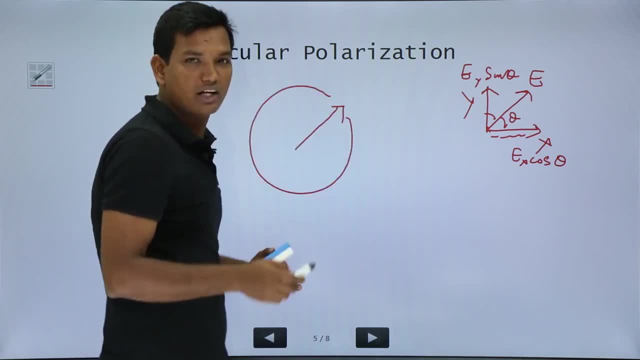 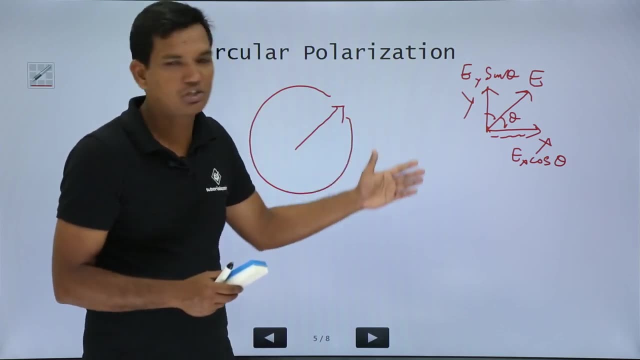 you rotate this field like this, okay, whatever the polarization or the pattern of electric field will be generated. that would be what is called as circular polarization. Let us look at the picture of this and then we will understand more on this. So this is what is your. 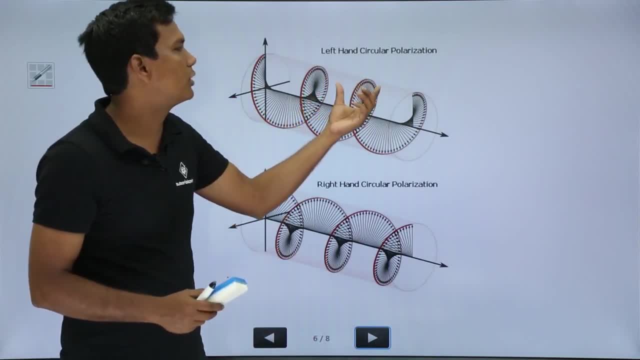 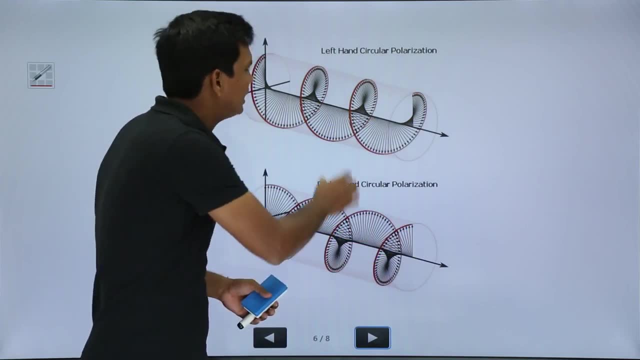 circular polarization. If you observe, there are two kinds of circular polarization is one is called as left-hand circular polarization, another is called as right-hand circular polarization. It is nothing, but we will see the left and right-hand later. Let us see how it is. 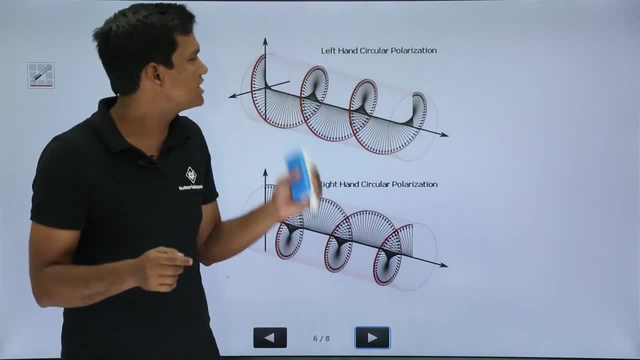 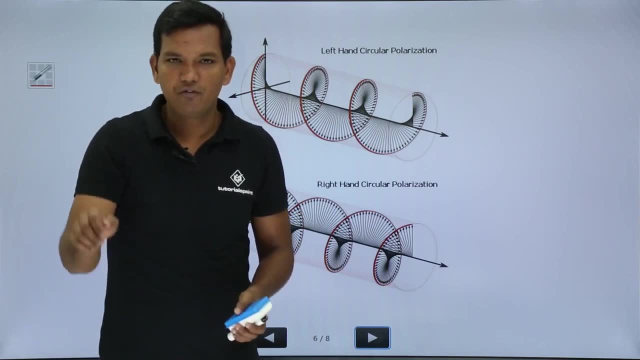 You see that if what I can do is I can understand the same polarization with the thread example right Now. previously in the linear polarization I was moving the thread like this right Or like this: If I start moving the thread in a circular, if I rotate my hand very fast like this, what? 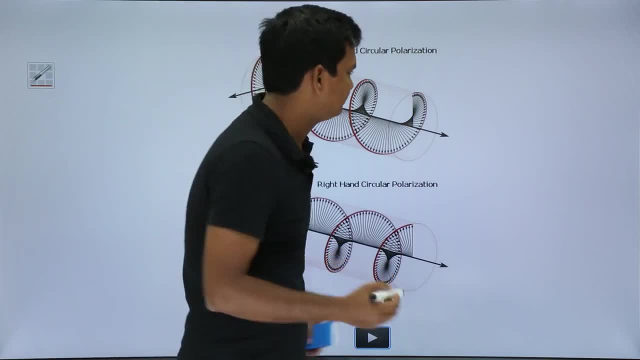 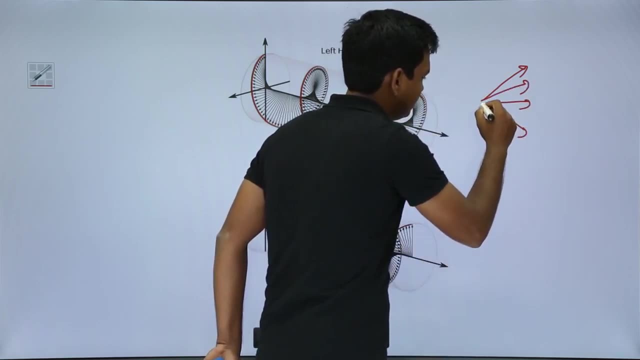 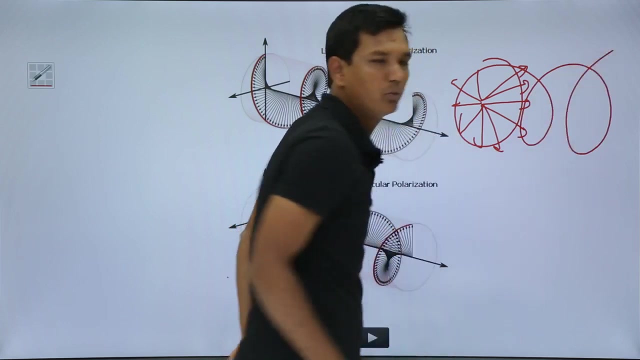 will happen. The thread will take the circular loop right. So basically, you take one field and you start rotating at every point of equal radius. This will be keep on rotating and this will be keep on going right, That is. it is a very easy. 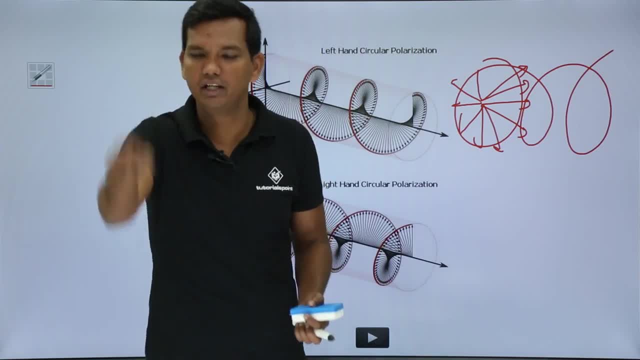 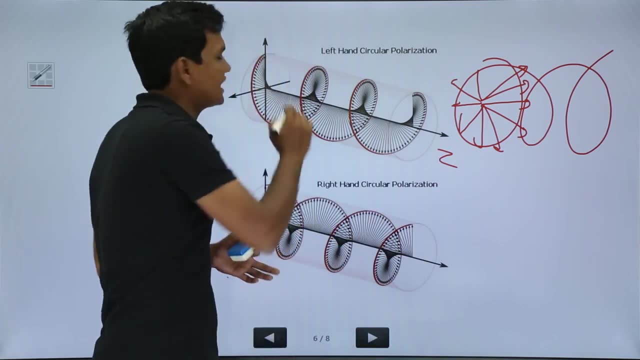 to understand with the thread. right, You keep on moving and the thread will be rotating and it will be going. So it will be propagating in some direction, but the variation of electric field will be not along the x-axis, It will be like this, You see. 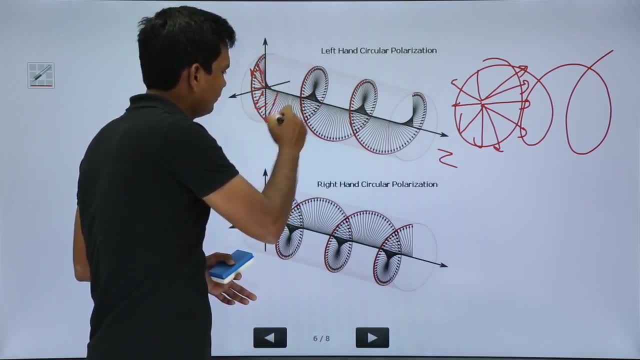 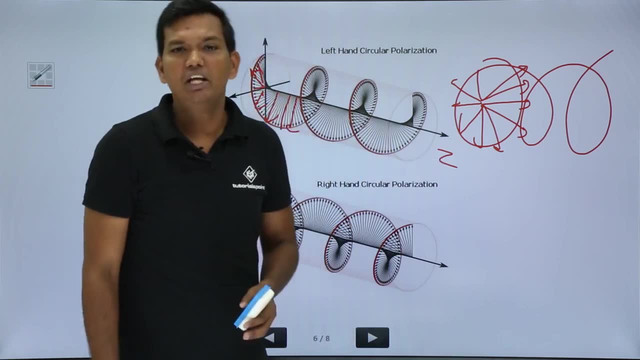 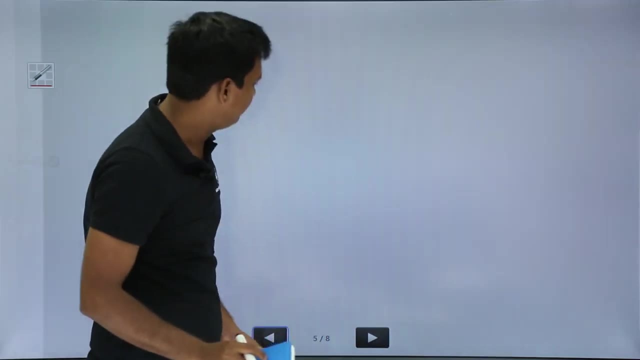 every point it is changing right. You can see that It is a circular right And it is going right. So this is what is called as your circular polarization In terms of equation. if I want to understand this, how can I understand that? If I want to go into equation form, 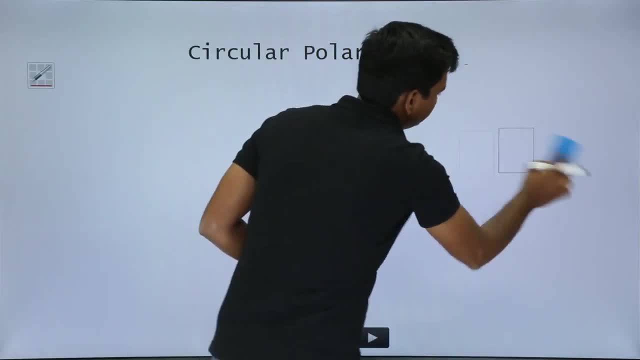 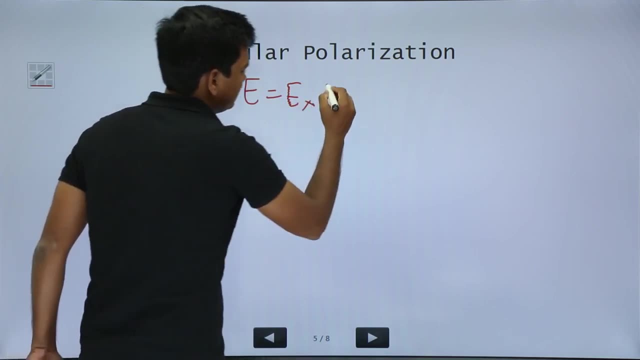 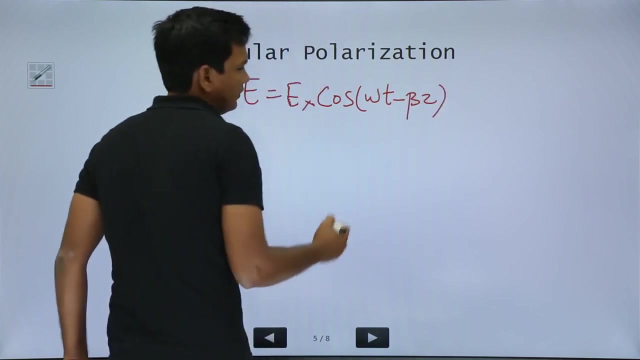 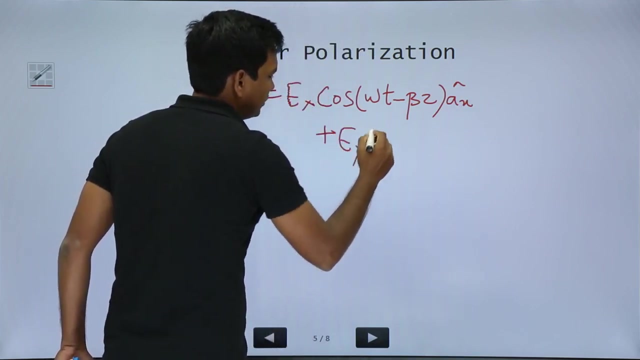 what I will do is let me rub this. So what I am going to do is I am going to write E field. E field will be nothing but E x. Let us say E x cos. omega t minus beta, z, A x cap. This is one Another will be. it will have plus E y cos. 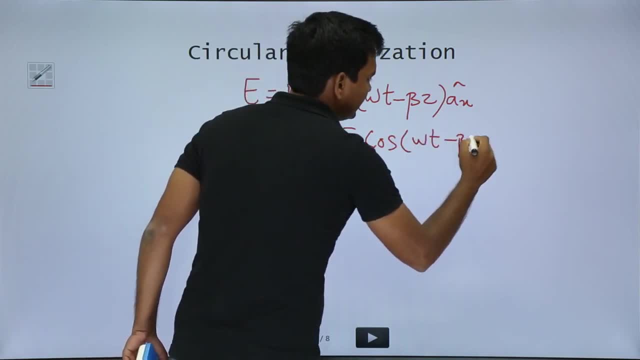 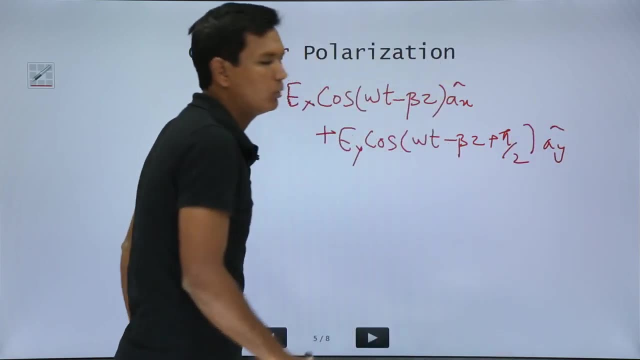 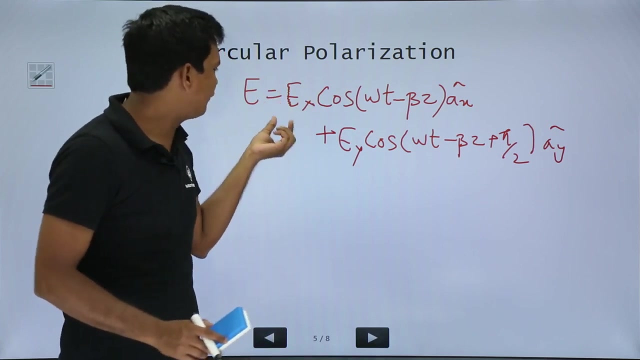 omega t minus beta z plus pi by 2 E y cap. Now what I have done. You see, this is one of the equation which actually nothing but which satisfy the circular polarization. Electric field has two component, E x and E y. The phase difference between x and y is 90 degree. 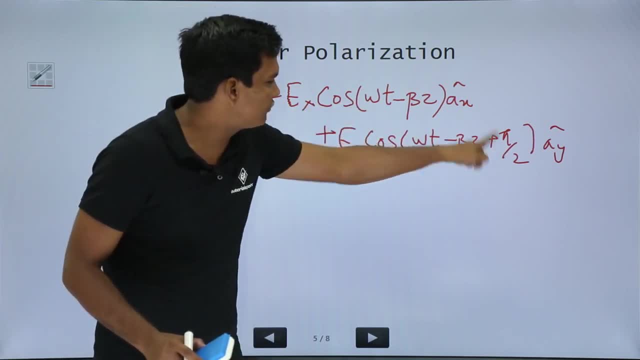 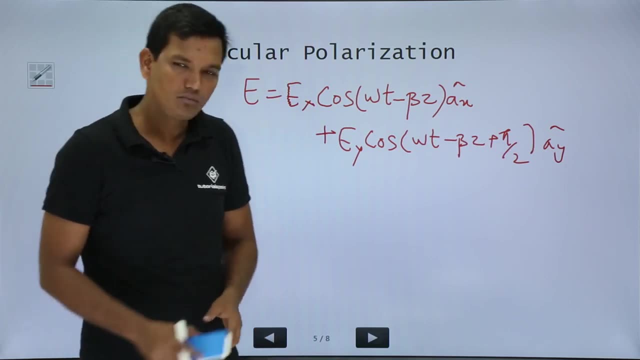 You can see that right This, between E x and E y there is a phase difference is pi by 2, which is nothing but 90 degree. One component is along the x-axis, another component is along the y-axis, right? So if that is the case, when your phase difference between the two components of 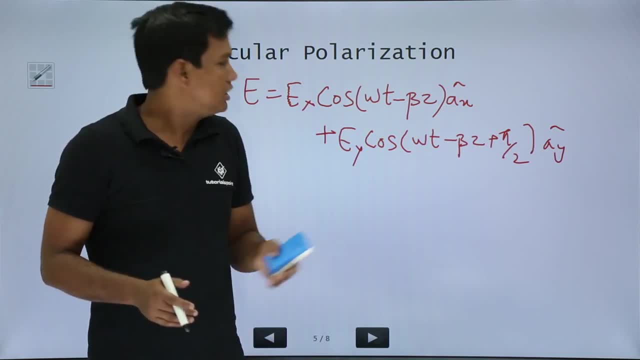 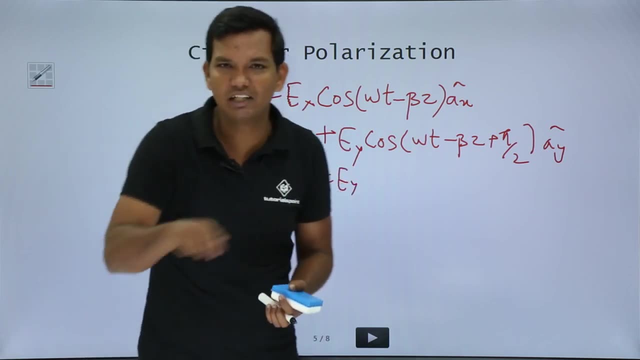 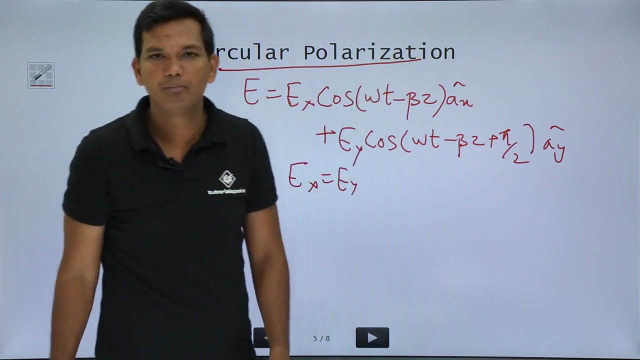 electric field is nothing but 90 degree and in that case, and also your E x should be equal to E y, right? If you want to make a circle, right, Then it should be equal radius, right, All the radius should be equal. In that case, this is nothing but your circular polarization right. So when you have 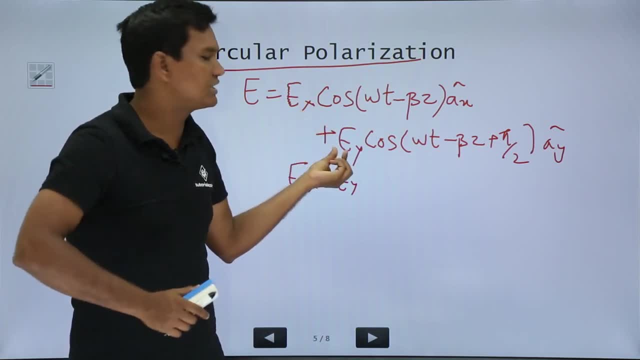 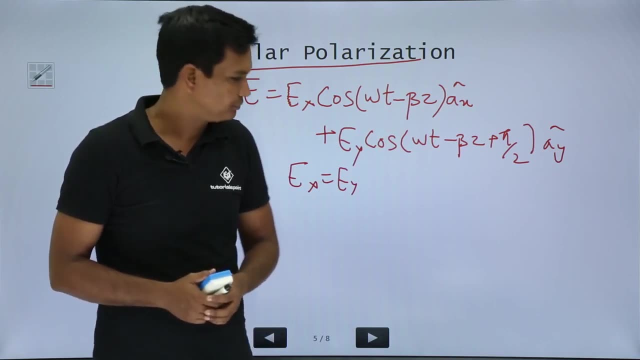 an electric field given. if the amplitude of E x and E y are equal and the phase difference between E x and E y is 90 degree, then it is nothing but your circular polarization. We will see the next type and the last type of polarization, which is nothing but the elliptical polarization. 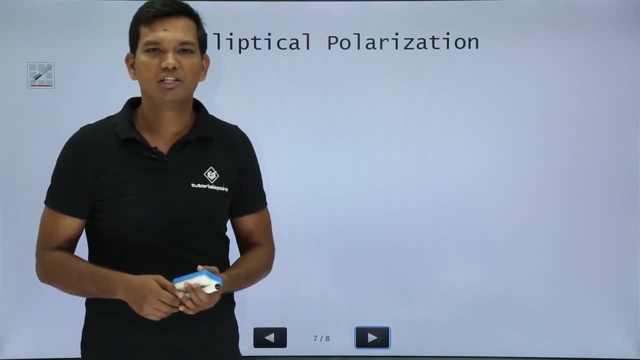 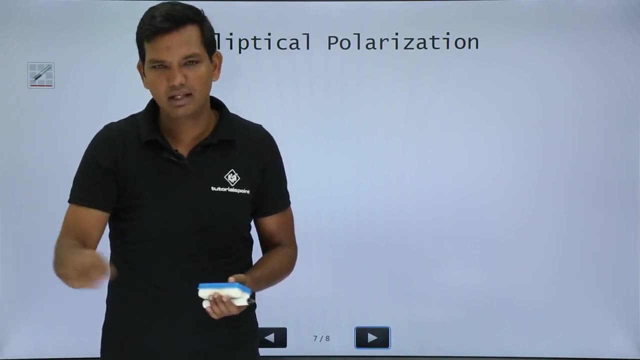 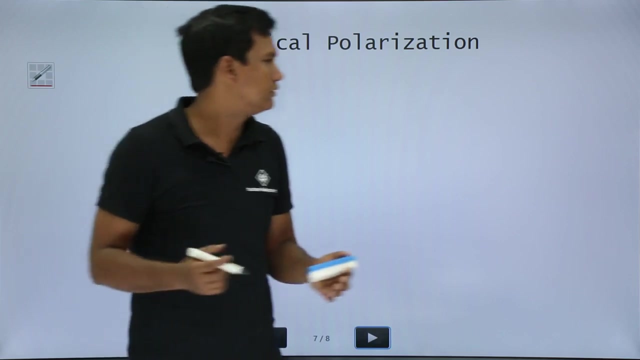 So let us come to elliptical polarization. What is the elliptical polarization? If I take away the same thread example, what I will do is initially I was moving the thread like this, and then like this, and then I started moving like a circle. Now what I will do is I will move the thread like this in such a way that in such a